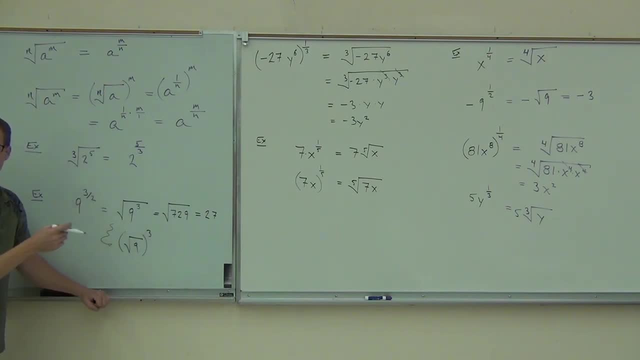 Q: Do you see that I just moved the 3 to the outside? Now watch, I'll bet you all can do this problem very simply. Can you tell me what's the square root of 9?? Oh, everyone answered. This is 3.. What's 3 to the 3rd? 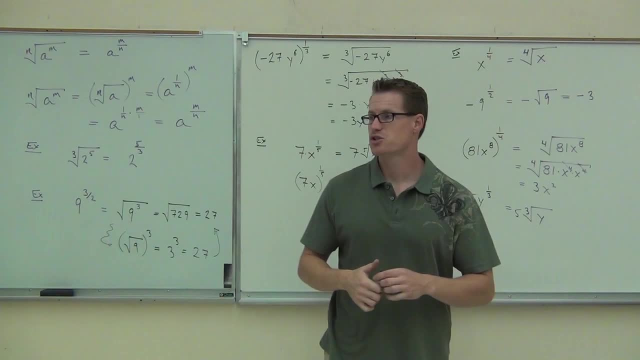 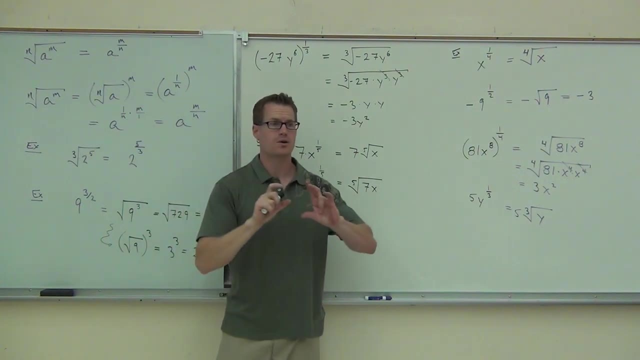 Was that a lot easier? Okay, so maybe a shortcut. That's not even a shortcut. You're just doing one step. that I told you was true. If you do that step and move the power to the outside, if you have to do these in your head, 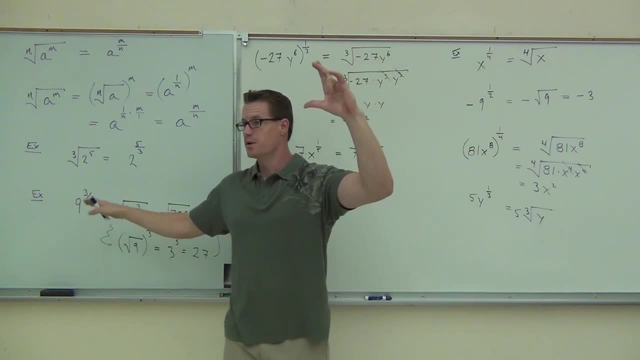 if you've got to do them in your head, the calculator will do this for you, no problem. But if you have to do them in your head, do the root before the power, if you can. You with me on that. Do you see why? 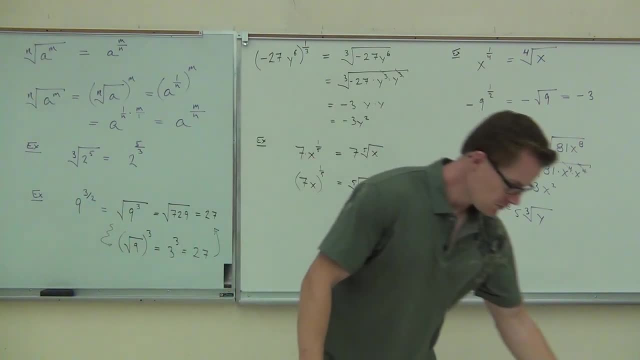 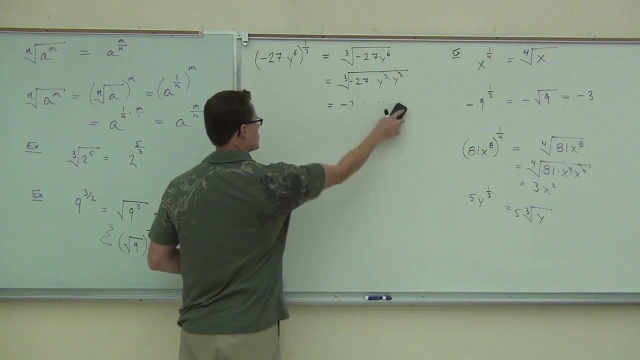 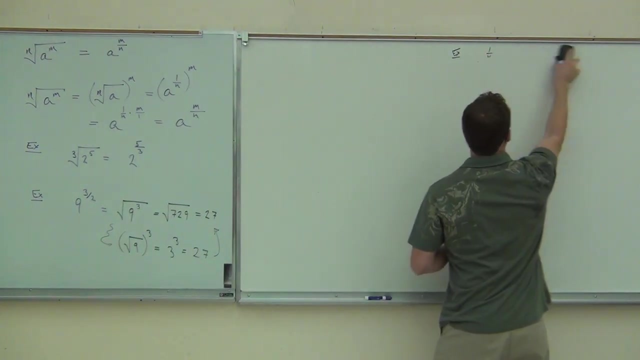 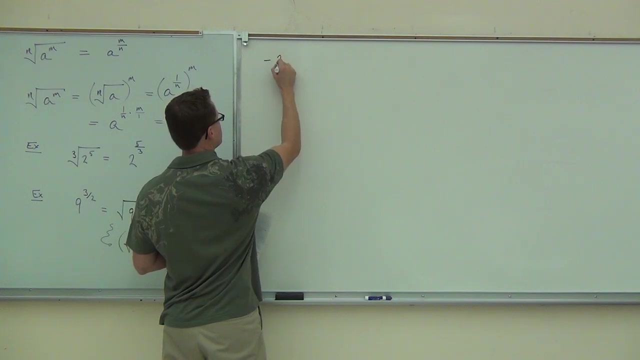 You don't want to do it with big numbers, right, Do it with small numbers first. Well, let's try a few more. Ultimately, I want you to be able to write the radicals very well, And then, after that, I'd like to see you simplify them. 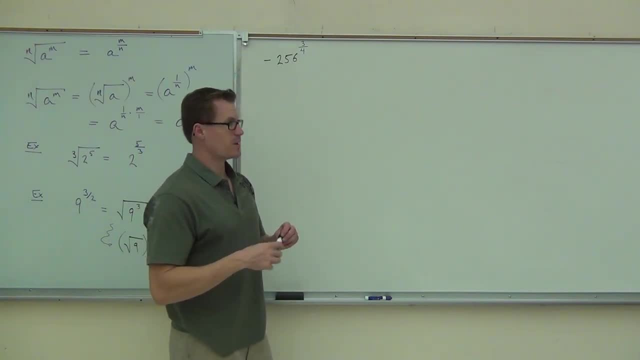 But first step, you've got to be able to write these correctly. So, everybody, what is the type of root that I have? Fourth root, great. Is the negative going to go inside the fourth root or outside the fourth root, Good, And do I have any power inside that root? 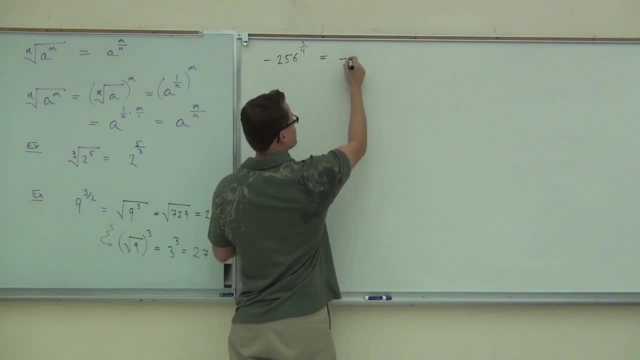 Okay. so firstly, I want to see you write it correctly like this: We definitely have a fourth root. Don't forget about that four. We've got a negative outside because it's not in any parentheses. We have a 256 to the third power on the inside of the root. 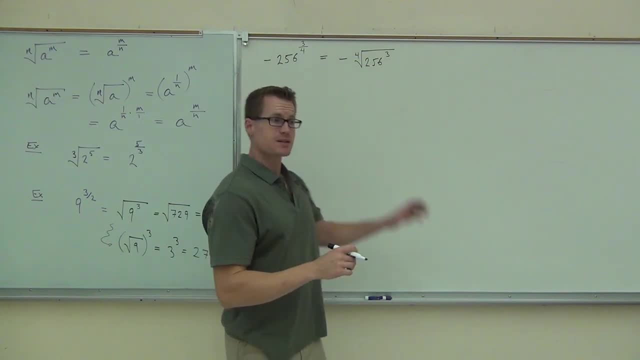 Not too bad if you're okay on getting that far. Next, try to simplify it. This is step one. I want to see that that you're able to do that, Because sometimes we're dealing with variables We can't just do. we can't do this process very well. 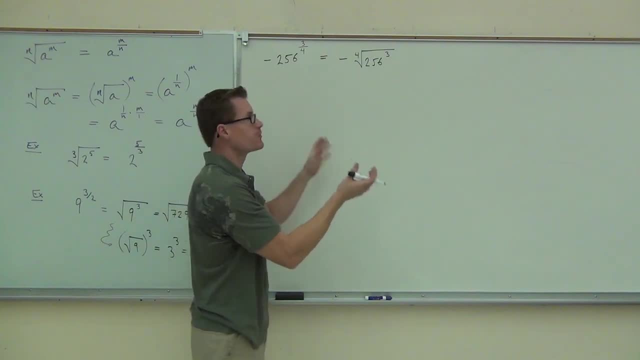 So sometimes we're not going to be able to do that. In this case we will, But firstly write it this way. Just make sure that you can. After that, do we want to take 256 to the third power first? 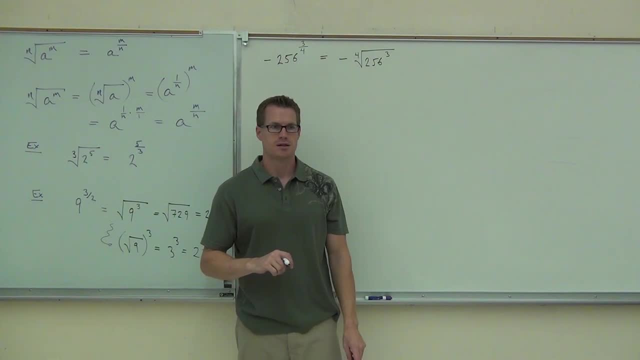 Or should we find the fourth root of 256?? You take 256 to the third power. That's insane. That's a really, really big number. That's huge. Instead, you could think of it as negative. Take the fourth root of 256 to the third power, like that. 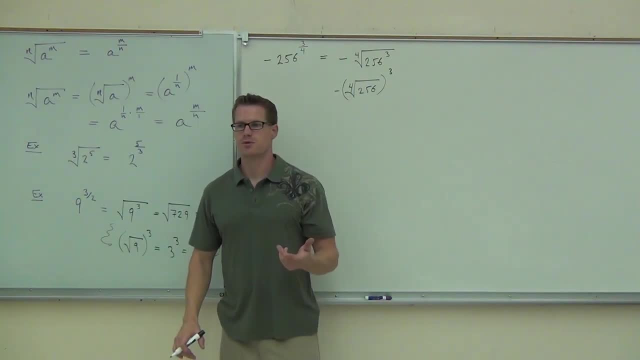 Take the fourth root first. Now, maybe the fourth root of 256 isn't popping right into your head, but it does exist. Say it now Four. Well, it popped into your head. It popped into my head too. It did, it did. It popped right in there. 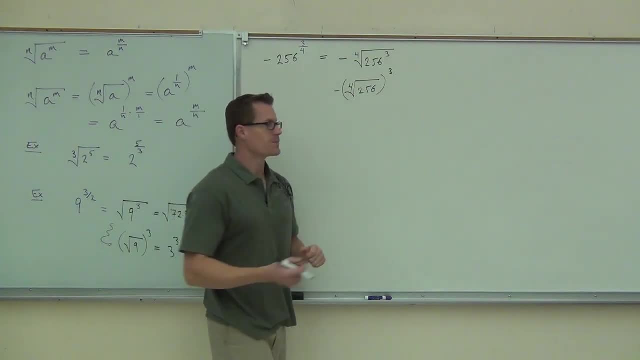 I promise. Yeah, it is, it's a four. So this would be negative. four to the third, Negative four to the third. What is negative? four to the third power? Well, we'd say negative. but how much is four to the third? everybody? 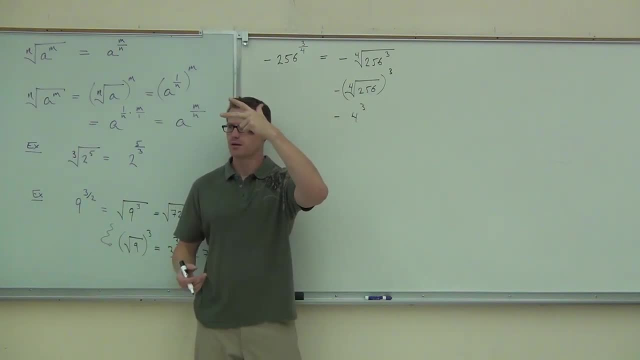 64. That's four times four times four right 16.. Four times four is 16, times four gives you 64. This is negative 64. So, step one: write the radical appropriately. Step two: try to simplify it. 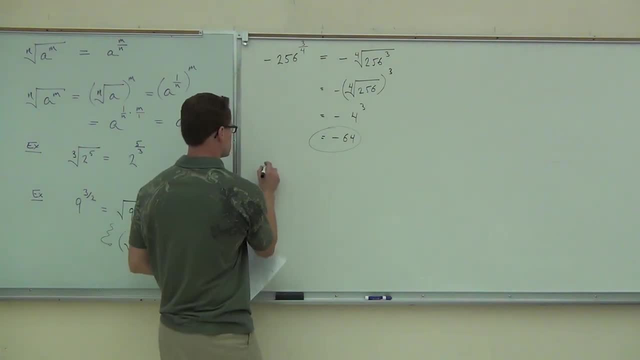 Let's do a few more of these things. Negative 32 to the two-fifths. We're going to go kind of quickly through this because we should have the root down at this point. What type of root do we have, folks? 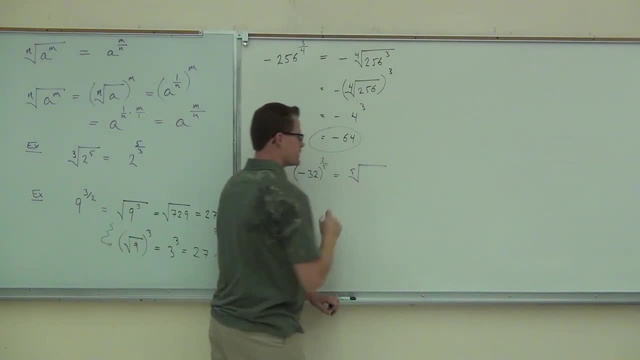 A fifth Good, So I'm going to have a fifth root. Is the negative equal to two-fifths? Is it inside or outside of the root, please? Inside, Inside, So I'll have negative 32.. In fact, do I have a power? 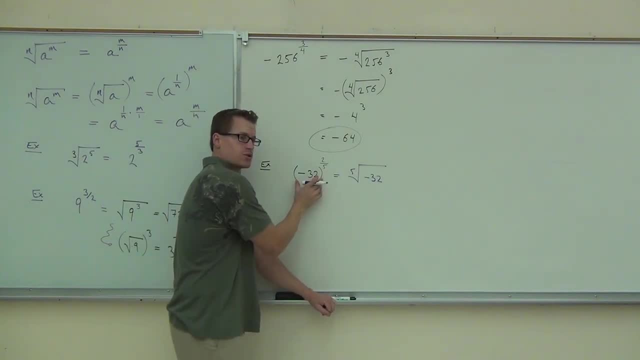 Second power. Second power Now, because this was in parentheses, I want you to watch up here on the board. Please watch. I'm not just going to put a two there, Right there, that two would not be applied to negative 32, it would just be 32 and you. 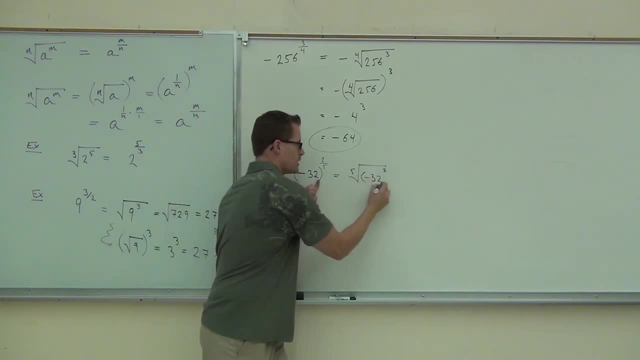 would take the negative. Are you with me on that? Because this had a parentheses. it really is a parentheses like that. That changes the problem a little bit. This is going to make whatever you have a positive number. Are you with me? 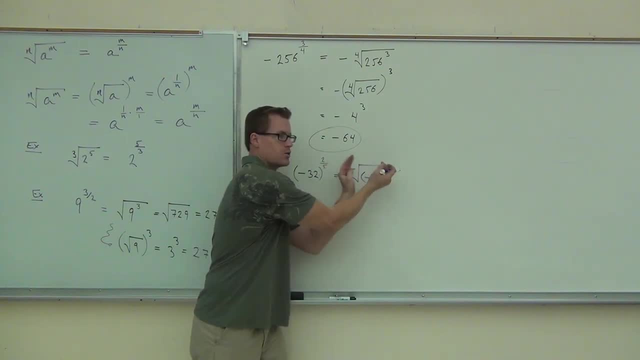 That's what that does. So you need that parentheses. If you have one here, you also have one there. Nod your head if you're with me. Okay, Good deal. Now we could square negative 32 and then take a fifth root, or you take a fifth root. 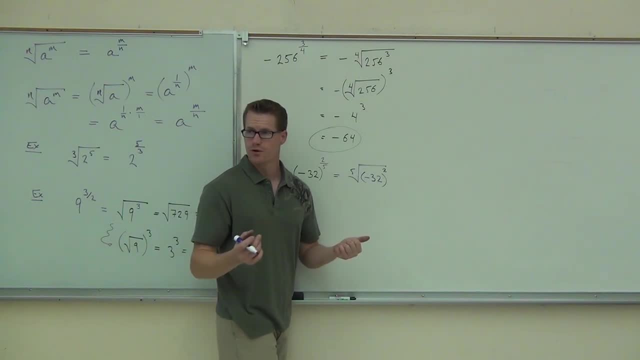 and then square. whatever you get out of that, I'm going to choose to take the root first. So if I take the root first, what I'm doing is a fifth root of negative 32 and then squaring it. Can you tell me what's the fifth root of negative 32?? 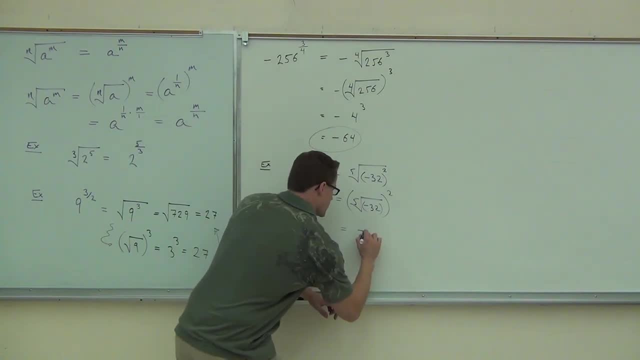 Negative 2. Negative 2.. Okay, I have negative 2 and then I'm squaring that number. Remember, I'm doing this part first, I'm doing the fifth root first and then I'm squaring it. It's negative 2 squared folks. 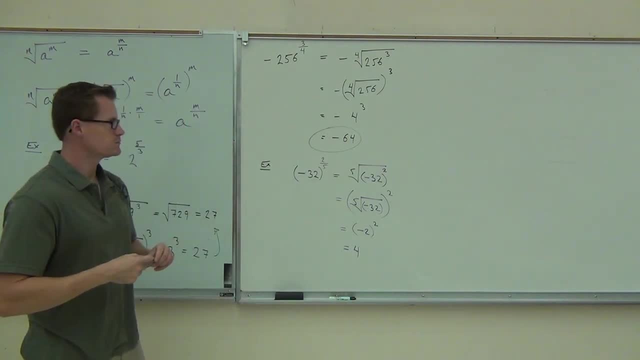 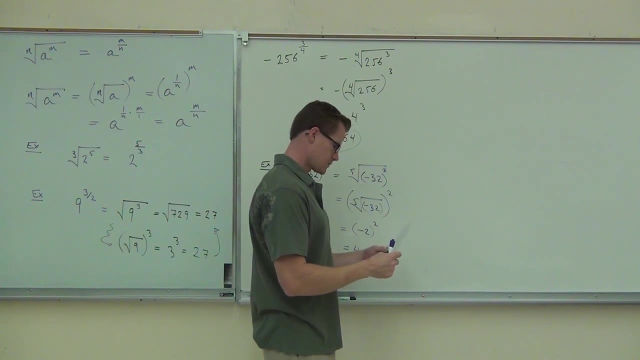 That's 4.. Let's try a couple more together. I'll give you one more. Okay, Let's try a couple more together. I'll give you one on your own. Then we'll move on to some negative exponents. Look at what happens there. 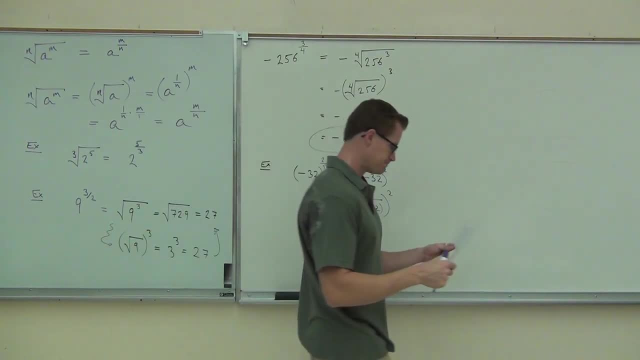 And after that we'll talk about some exponent rules to refresh your memory a little bit. Okay, You knew this was coming right. We're dealing with fractional exponents. How about a fraction to a fraction? You're crazy, Leonard. 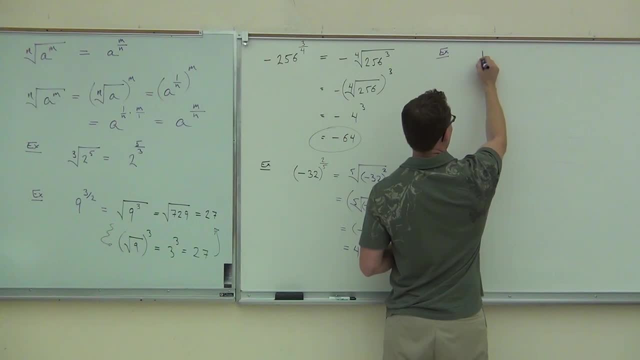 Come on, What are you doing to me? A fraction to a fractional exponent? I didn't know this was a math class. Come on, It's only 735.. My goodness, Yeah, What about a fraction to a fractional exponent? You're crazy, Leonard. 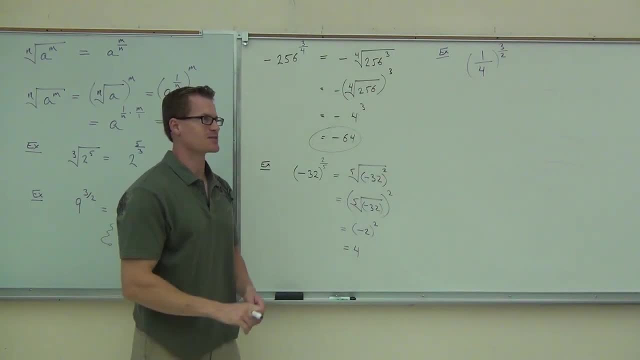 Come on, What are you doing to me? A fraction to a fractional exponent. I didn't know this was a math class. You're crazy, Leonard. Come on, What are you doing to me? I didn't know this was a math class. 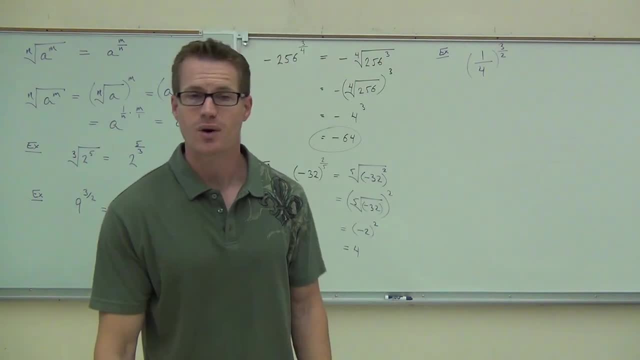 You're crazy, Leonard. Come on, It's only 735.. My goodness Yeah. What about a fraction to a fractional exponent? My goodness gracious. Well, what we know about fractions is that we take the top to that exponent and the 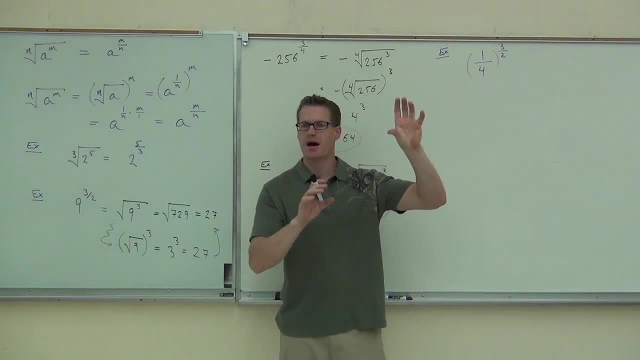 bottom to that exponent, the numerator to that power and the denominator to that power, and we solve the right thing. So you could go about and you could write this as: what type of root? A square root of 1. fourth to the third. 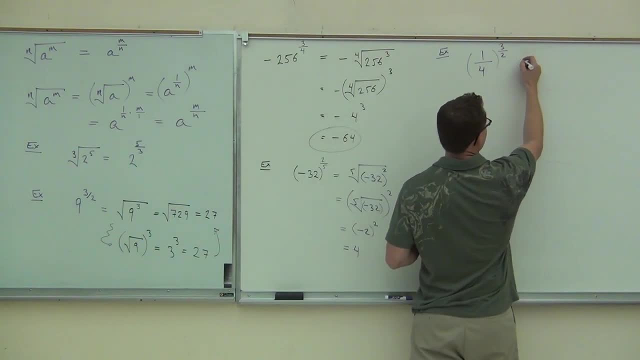 That's appropriate. That's appropriate. Well, what that means is that you can write this as a square root of 1 fourth to the third. That's okay, too right? Can you take the square root of 1 fourth? How much is it? 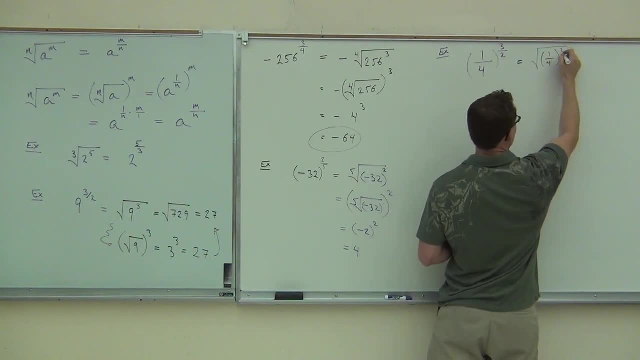 One half. Okay, So this process still works with fractions. No big deal. We're going to have 1 half, 1 denominator, 1 fourth, 1 denominator and 1 fourth, and we're going to write that as what type of root. 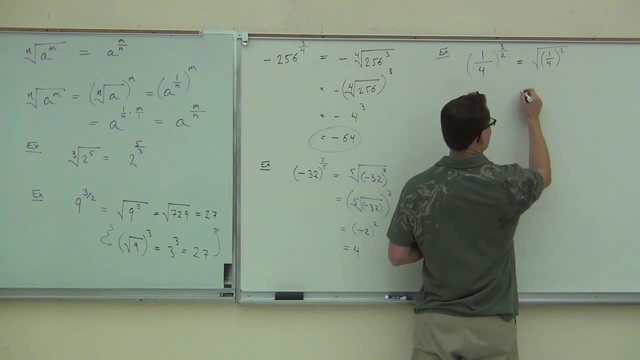 Square root, Square root of 1 fourth to the third, One half. So that's the relationship. There's no subtraction. That's the equation. So you're going to solve the problem. We have a fraction to a second. We're going to do it again. 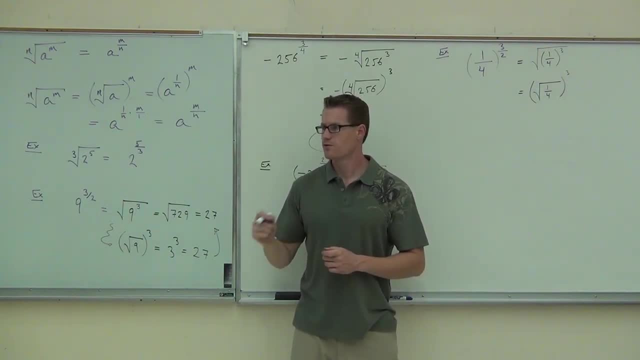 So we're going to go back and write this as something that we'll just make a little second. Well, that's right. It's 1 over 2, right? So I'm going to use this. How much is it? One half. 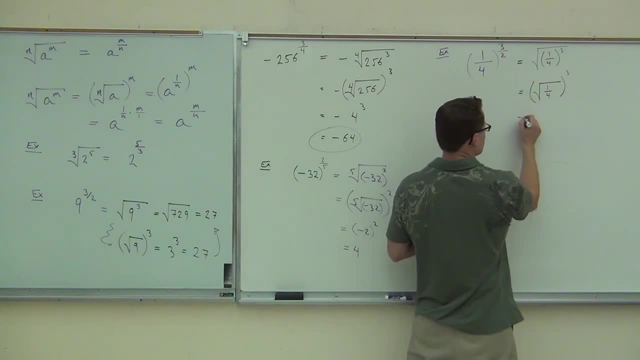 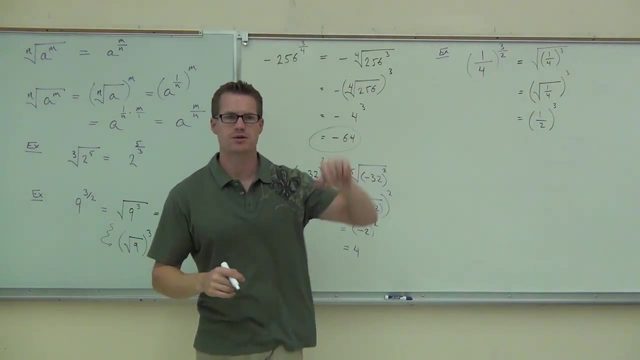 Okay, So this process still works with fractions. No big deal. We're going to have one half, then take that to the third power. We can do one half to the third power, take the numerator to the third, take the denominator to the third. 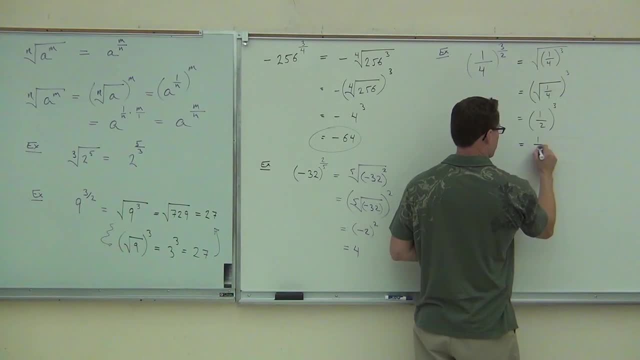 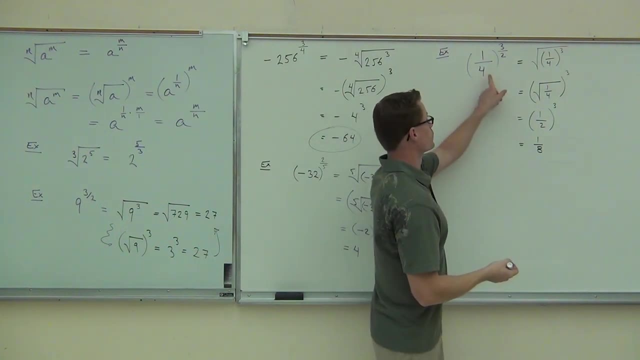 What's that? fraction One, even eight, That's it. So even though we have some fractions up here, no big deal, The same process works. We still know it's power over root. Whatever root we have is going to be on the denominator. 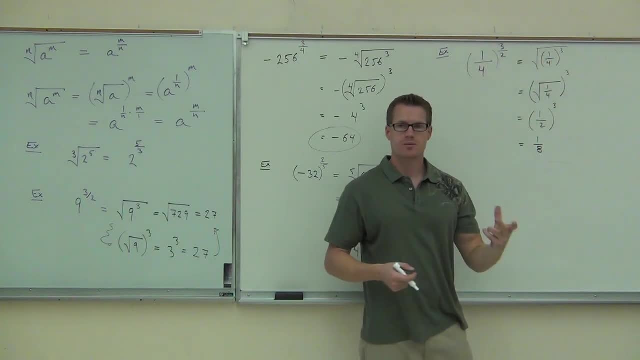 Whatever power we need is going to be on the numerator. Write it out appropriately and then use what you know to simplify that. Okay, One more before I let you go and do one on your own. Let's say we have 2x plus 1 to the 2 sevenths. 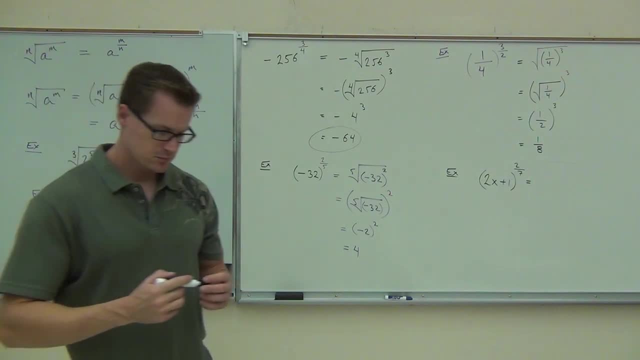 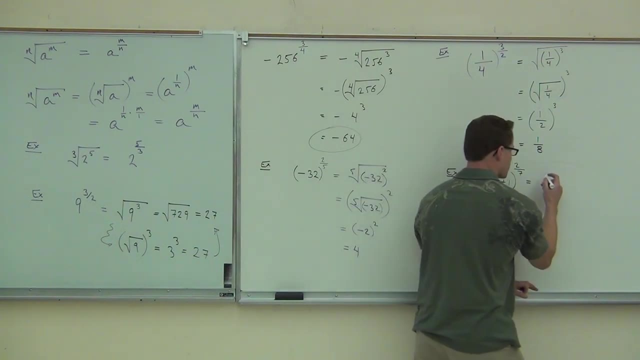 2x plus 1 to the 2. sevenths power. Ladies and gentlemen, what type of root do I have here? 7th root, And it's all in parentheses, So everything's going to be on the inside of that 7th root. 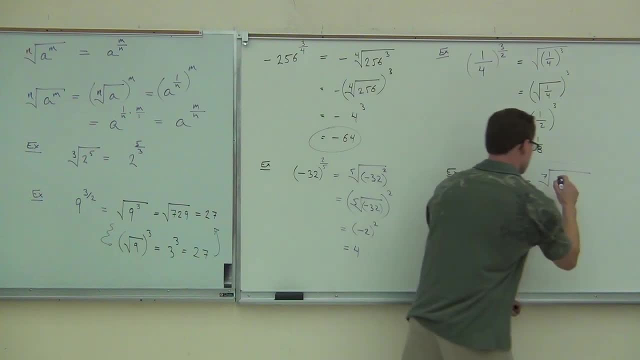 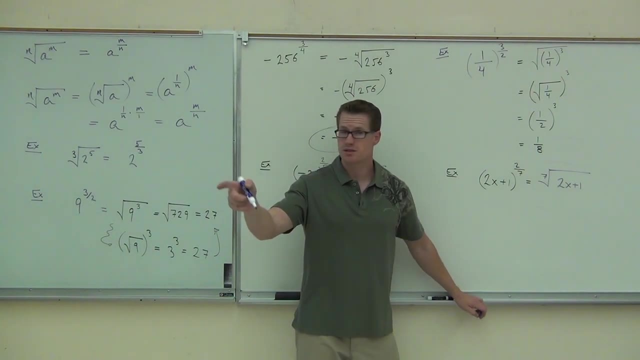 What is going to be on the inside of that 7th root 2.. Okay, Do I have any power associated with that? Parentheses and square root Parentheses, because, well, this was in parentheses and it's being squared. 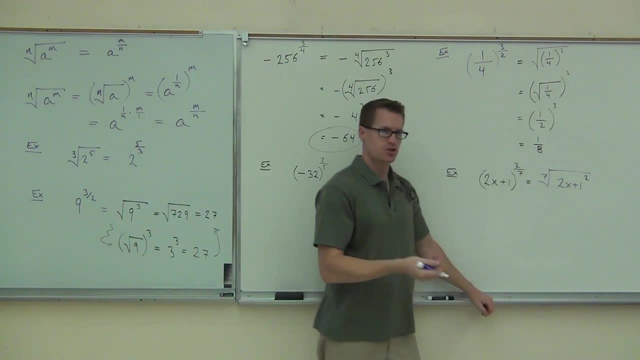 So I can't just do this. That doesn't make sense, right? That's just squaring the 1. What I want to show is that the whole thing is being squared. Put some parentheses on that thing, You're done. You can't simplify this one. 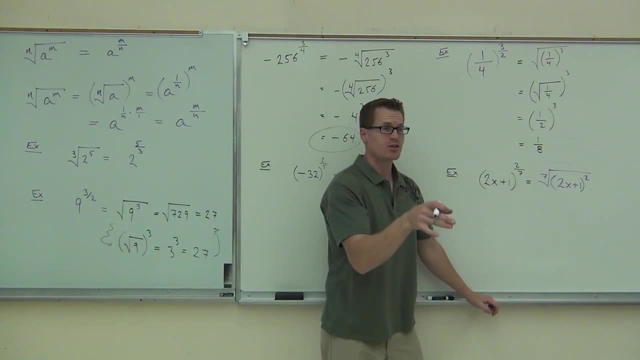 It's not like the other ones. I mean, if I say, okay, find me the 7th root of 2x plus 1, you're going to go. well, what's x? Well, I don't know. 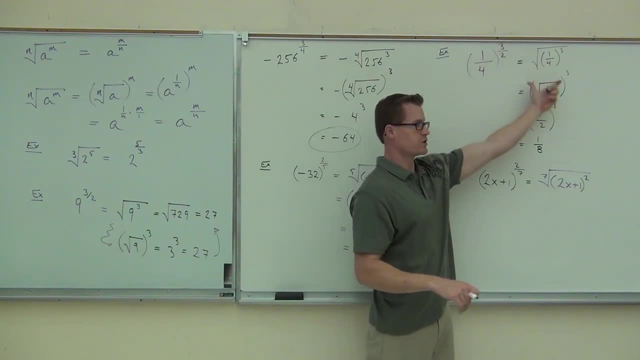 So we can't do anything with that, Right, It's not like the numbers. Numbers, yeah sure, We can just simplify those down Once you get the variables. really, there's only a select few things we can do, which is: 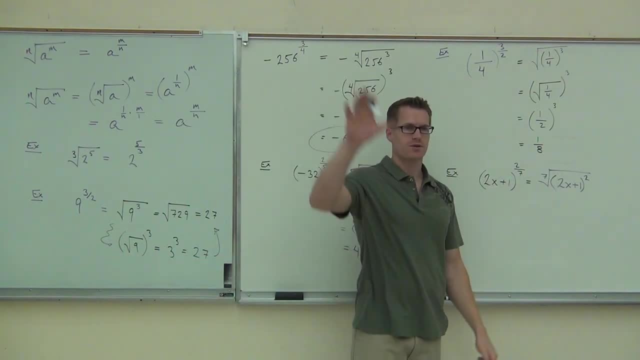 kind of nice. I guess that you're done at this point. Raise your hand if you feel okay with what we talked about so far, Good deal. I want you to try one of these on your own. Let's do negative 81 to the 5th. 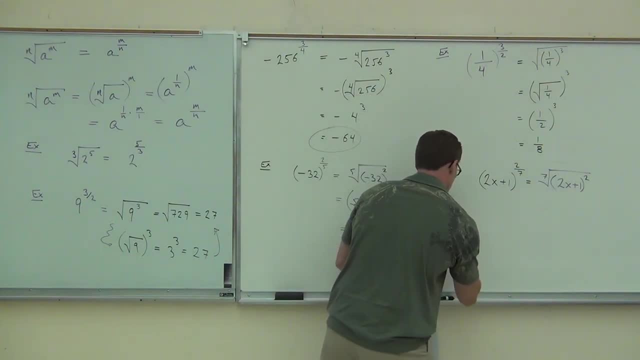 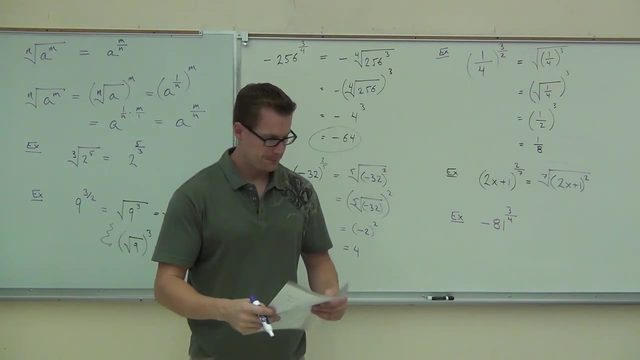 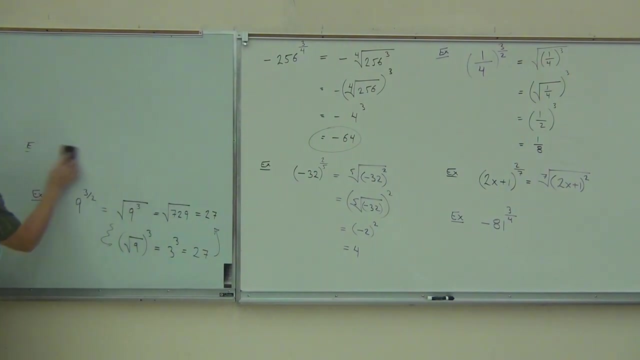 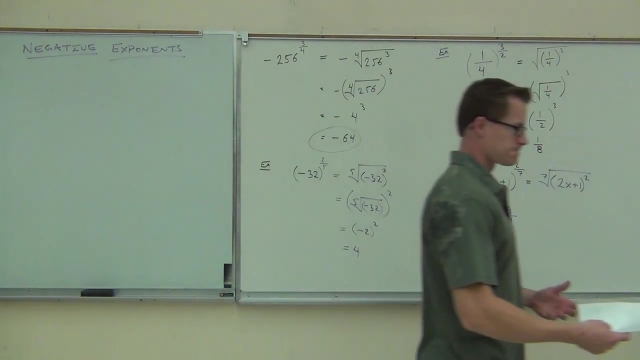 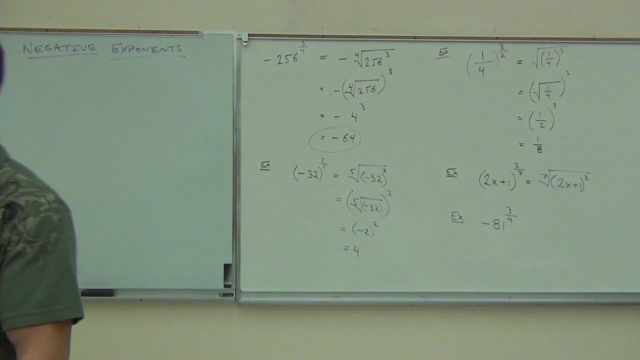 Negative 81 to the 3 4ths. Like that. Negative 81 to the 3 fourths. oh my, Did you find the root? What type of root? Fourth Good: Is the negative inside or outside the fourth root? 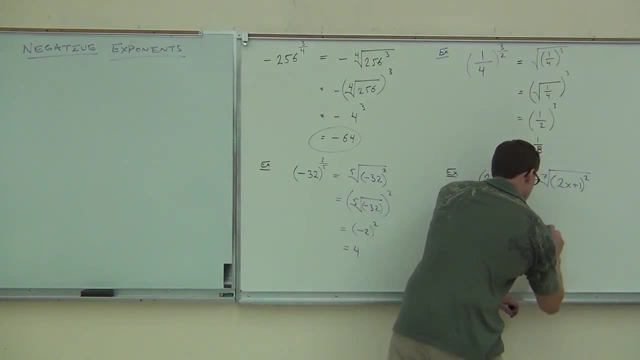 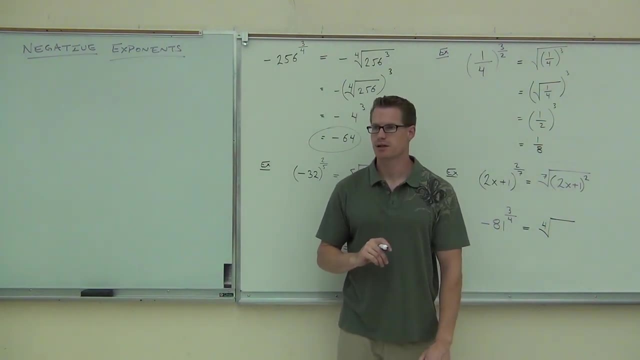 Outside. You know that's probably a good thing because if you noticed it, if the negative was inside the fourth root, that would be a problem, right? You can't have a negative fourth root. Inside we have our 81, no negative. negative is on the outside. but that's to the third. 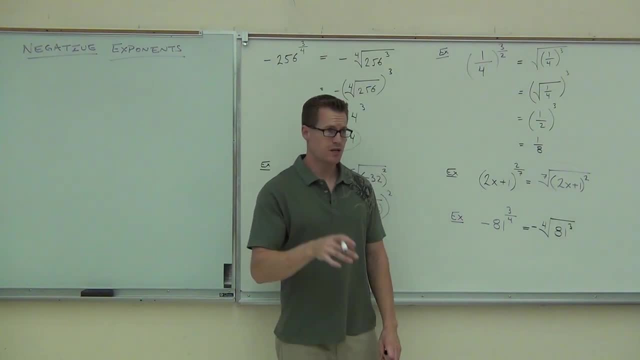 power. Now you can do this two ways. you can either use your calculator, find 81 to the third power and then take a fourth root- that's fine. Or you can do the fourth root first and then take it to the third power, and that's the. 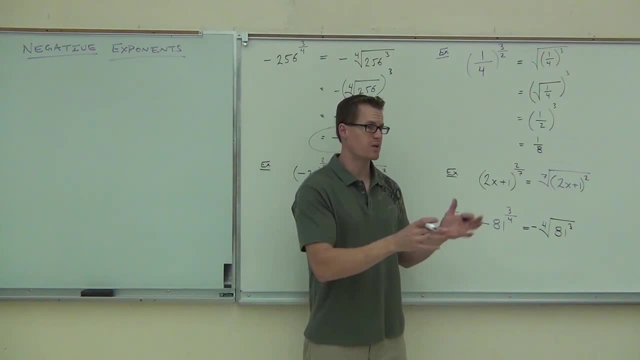 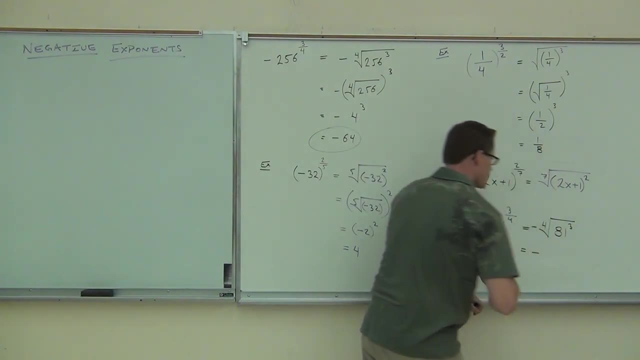 way we do this in our head You deal with smaller numbers. you make it smaller before you make it bigger. You make it bigger before you make it smaller. that's harder. So we'll still have the negative. we'll do the fourth root of 81,. what's the fourth root? 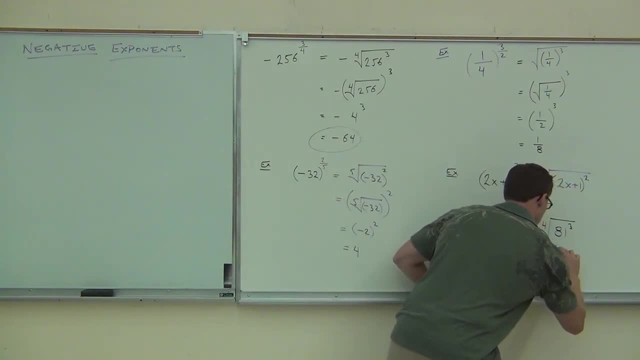 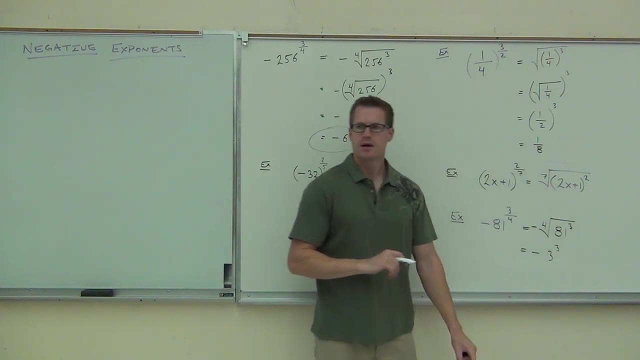 of 81? 3.. So we have 3 to the third power. Remember taking the fourth root first. that's the 3, we still have the third power. Is the negative being taken to the third power or just the 3?? 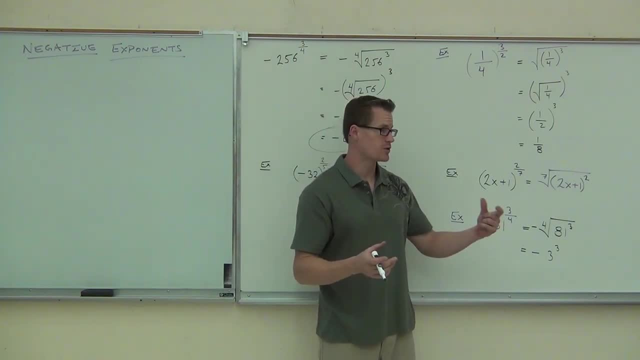 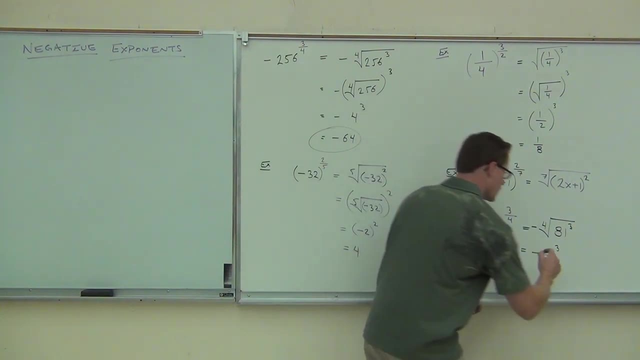 3.. Now, in this case it really doesn't matter, right? because we have the third power. so if you did negative 3 times negative 3 times negative 3, it's going to work out the same as negative 3 times 3 times 3, but I want you to understand the whole process here. 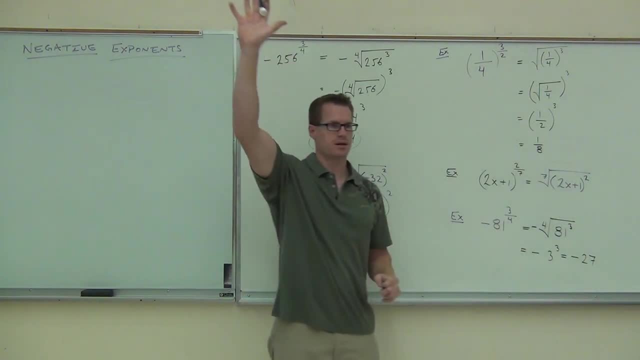 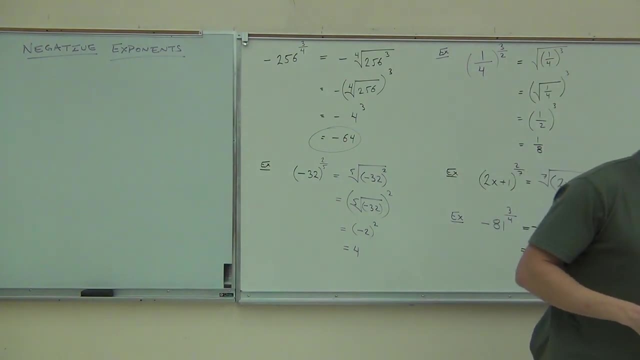 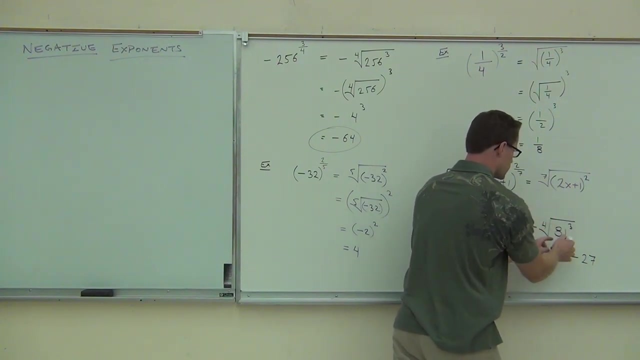 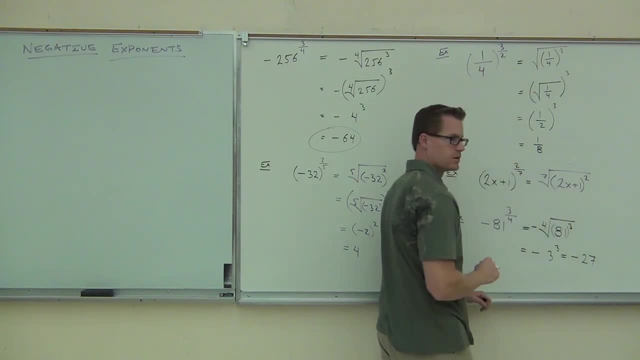 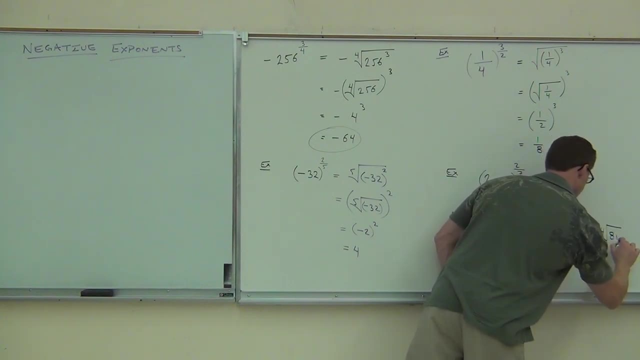 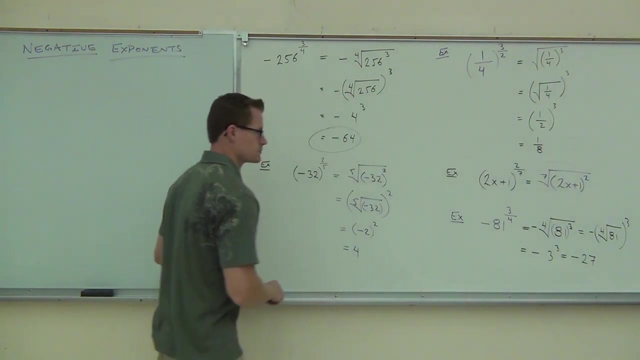 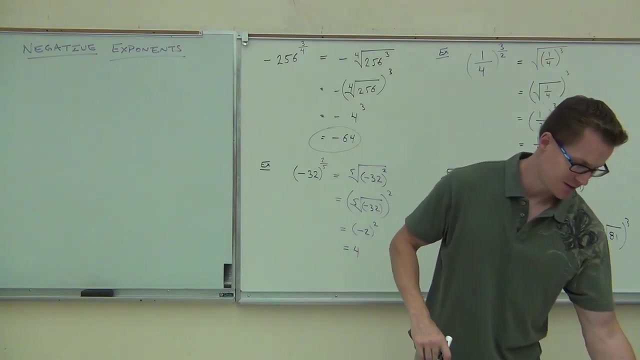 You could have done this. I didn't. I actually didn't show this step. I didn't show, I didn't show that step, but that's what we're actually doing. Okay, have we dealt with negative x once in this class? 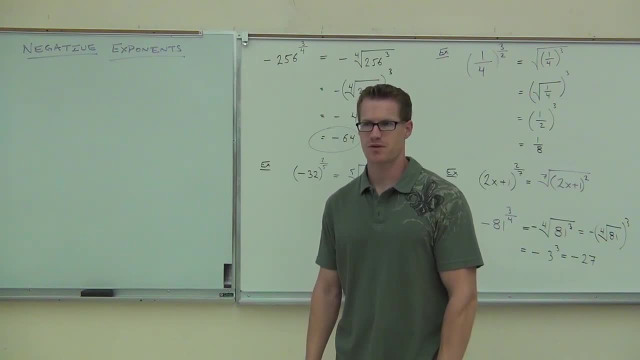 We did, briefly, I think. Remember, I gave you those problems where it was like complex fractions. you had like x to the negative 1,, you had 3y to the negative 2, and you did some crazy stuff with it and 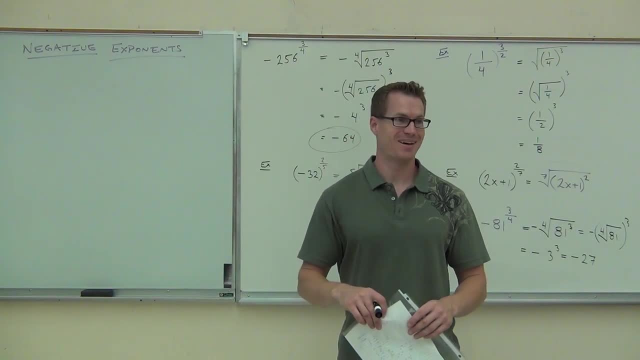 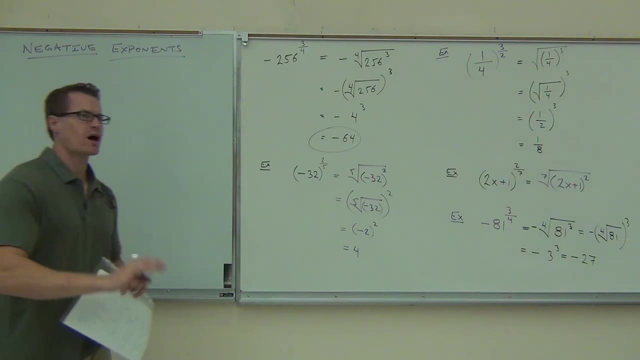 then it was like a 10-step problem. You remember those. Those are super fun, right? Obviously, Yeah, Well, we can still deal with negative exponents, even if we have some rational exponents. So negative fractional exponents, let's do it. 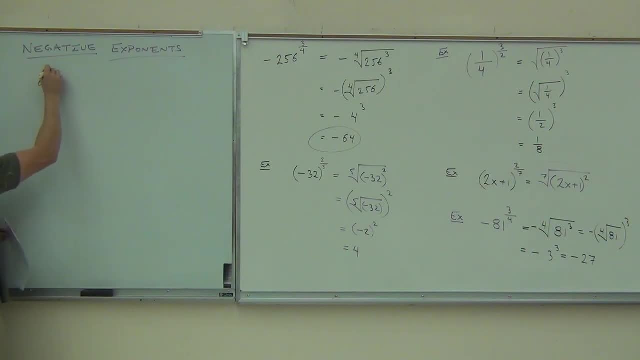 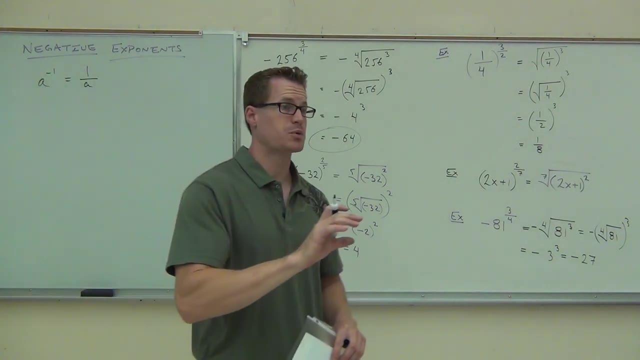 If you remember, a to the negative, 1 was the same thing as 1 over a. Do you remember that? That when we have a negative exponent, the way we change it to a positive is just put it on the denominator of fractions or essentially change it, change the position where it's. 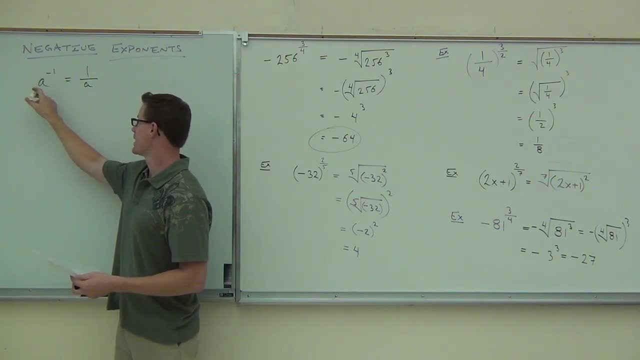 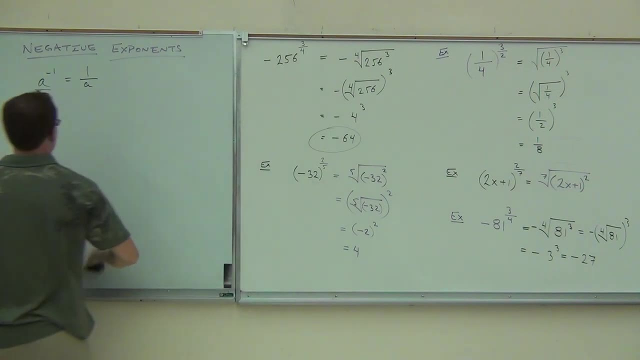 at. If it's negative on the numerator which it is here, remember this is like a to the negative 1 over 1, we move this to the denominator. That's, that's what we would do. We would spend a lot of time doing that. 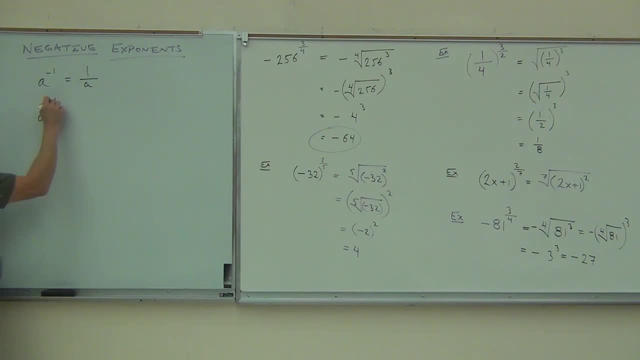 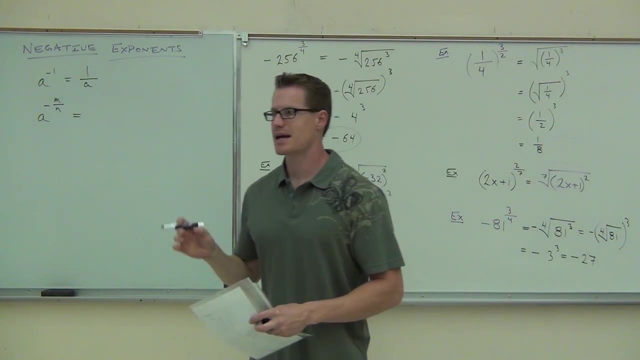 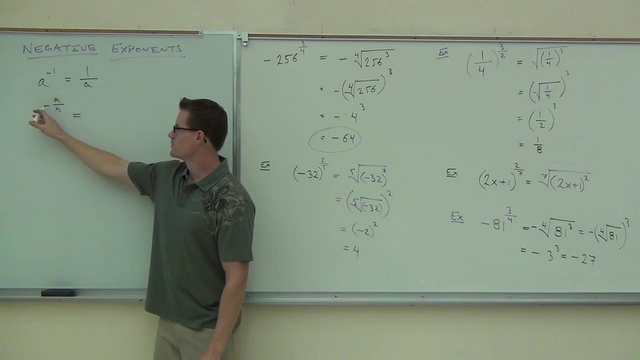 The same thing happens. if I have a to the negative, 1 over a, A to the negative, m over n, If I have negative m over n, what that says is that I have a negative exponent. Let me be real clear here. This negative has nothing to do with the sign of the number. nothing to do with that. 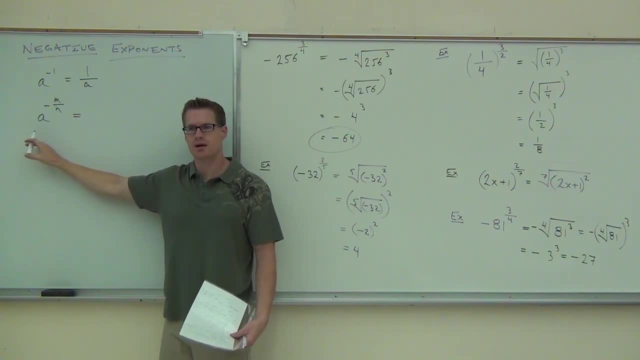 This answer does not have to be a negative. when you're done, I don't think you'll be okay with that. This doesn't have to do with the sign of the number. This just says that this is in the incorrect position. This is on the numerator, when it should be on the denominator. 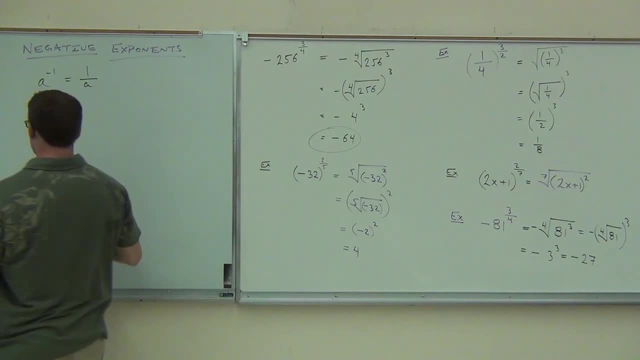 Okay If you want to make it positive. So what this says is alright. if I want to change my exponent to a positive, I'm going to have to move this from the numerator like it's on to the denominator. I don't flip anything around. I don't change the exponent, I'm changing where that that.